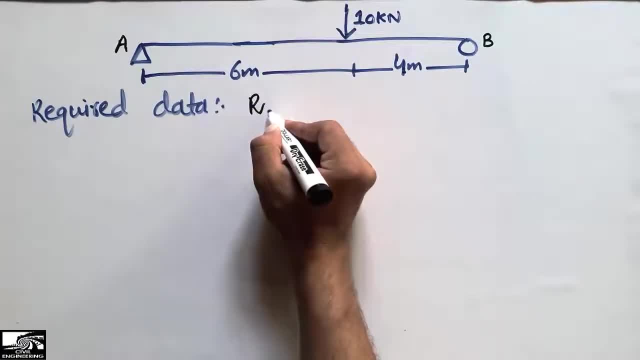 is to find the RA, the support reactions at A and the RA be the support reactions at point B, and we will also be refining that is, our support reactions are correct or not, by a vertical equilibrium rule. so to start the calculation, so let's consider this: the hinge support- here it's shown, of the 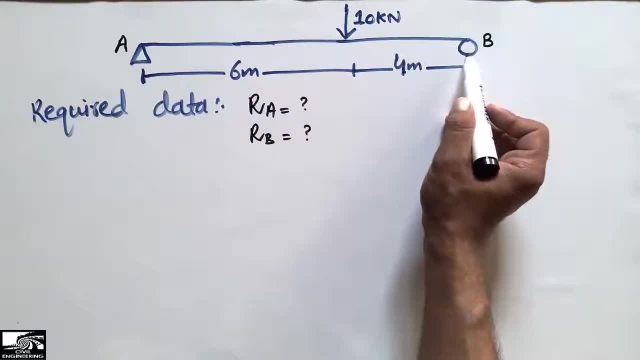 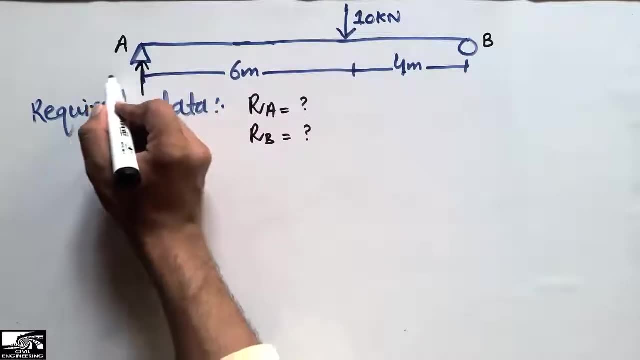 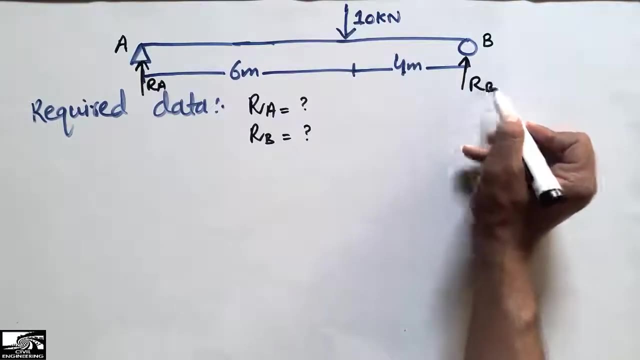 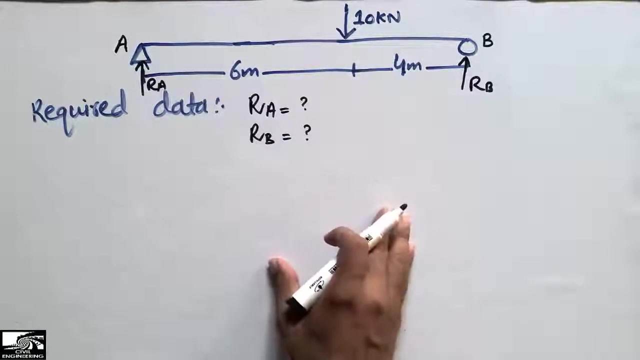 beam and this is the roller support, and these both are supports- cannot resist any moment. so, considering this at a point below the R a reaction, R a- right, well, it B point, we will have the reaction r B to support this concentrated load. the origins will act in the upper direction. now to start the 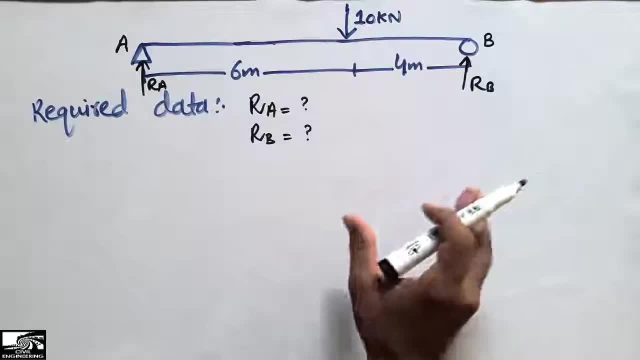 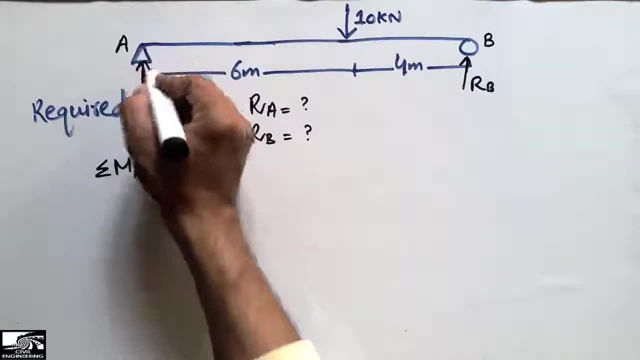 calculation. both these supports do not resist in a moment, so we can say that let's suppose the movement at the point is equal to zero, as the describe on the right side of the column are all impressionable. in this case The total moment at the point A is equal to 0.. 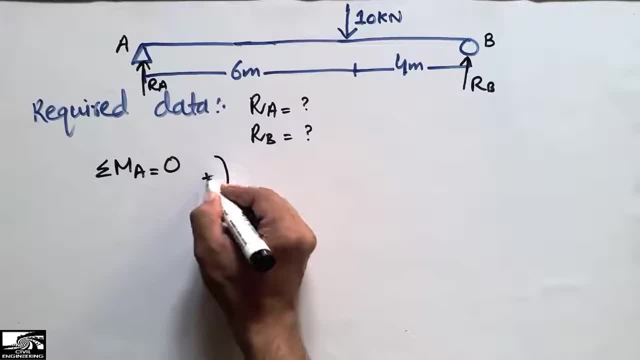 So in taking, the clockwise moment is positive, right, And the anticlockwise is negative. So when we have clockwise moment, we will take it with the positive sign And when we have anticlockwise moment, we will take it with the negative sign. 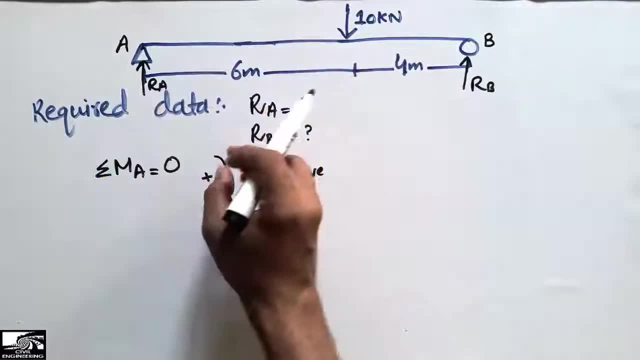 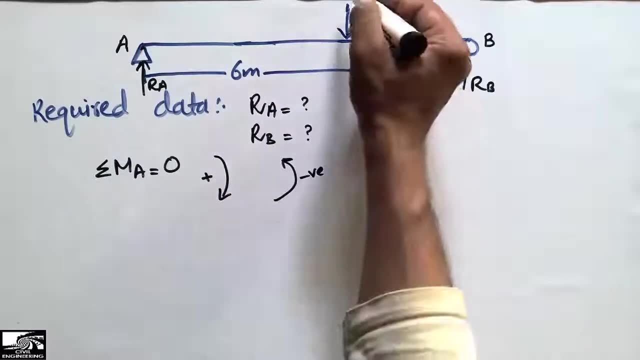 So summation of moment at A is equal to 0.. Now all the moments acting at point A we will calculate one by one. So the first one is the 10 kN which is acting clockwise. You can see here it is acting clockwise around the point A. 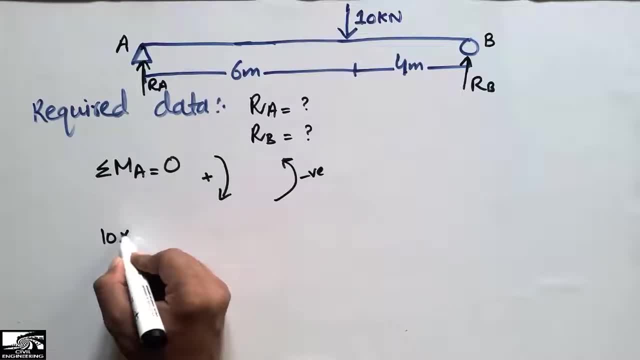 So the 10 kN is the force into the moment arm. The moment arm for this is the 6 m. So 10 into 6, here acting the moment at point A, And 6 m is the moment arm. 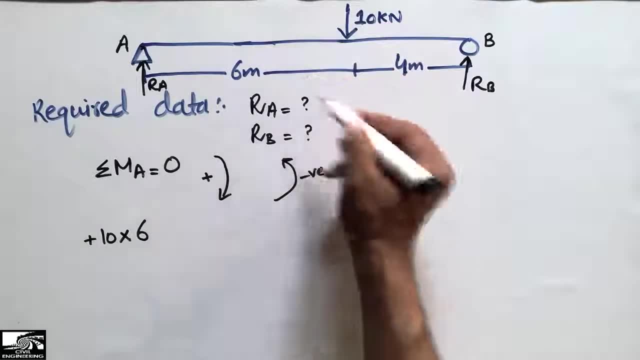 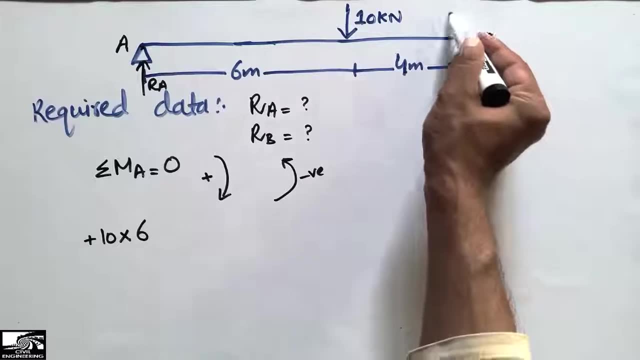 It is clockwise direction. so we can see it with the positive sign right Now. the other one is Rb. It is acting around the B. It is an anticlockwise sign. You can see here. it will act anticlockwise around the A point. 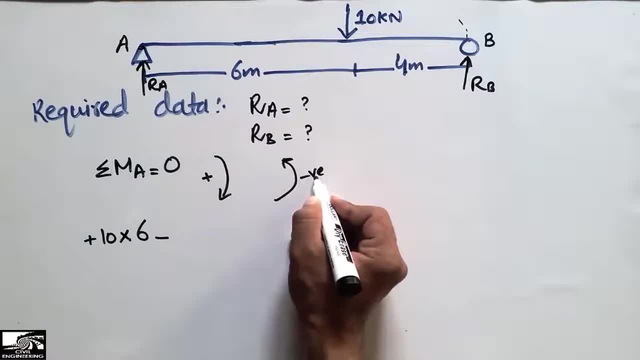 So we can write it here with the negative sign B, because we choose it with the negative. We assume that the negative moment will be a negative sign. So minus Rb into the moment arm. The moment arm is 10 m. you can see here from the B up to the A. 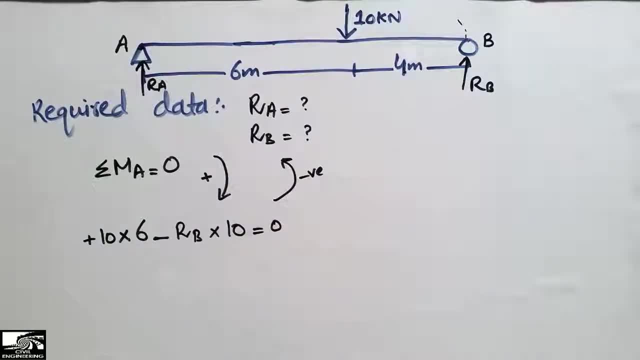 And the summation of moment is equal to 0,. right Now I will transfer this value to the right-hand side, so to get the value of Rb. So 10 into 6, 60 is equal to the 10 into Rb. 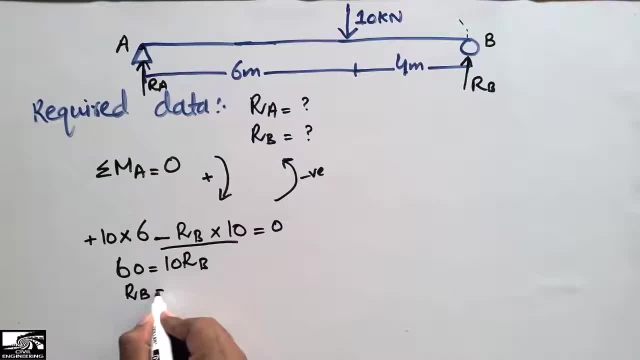 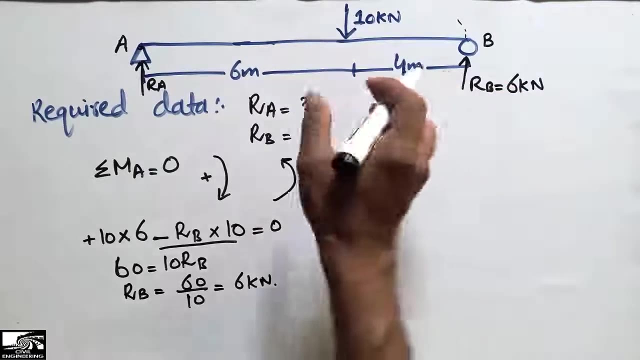 And we can write it here that the Rb is equal to the 60 divided by 10.. If we divide this 60 by 10, we will get the Rb, which comes out to be 6 kN. So it means that the Rb provides the 6 kN load resistance to this load. 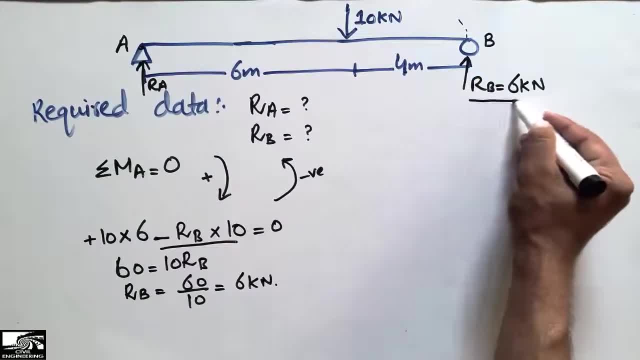 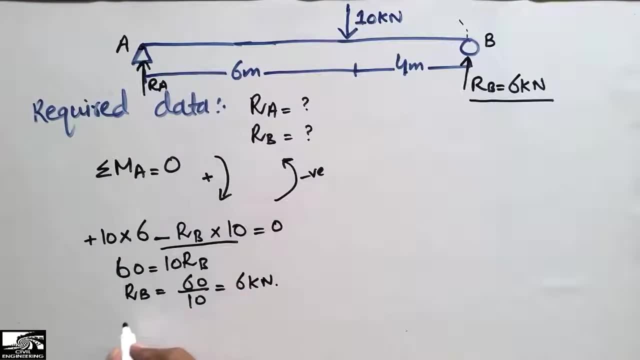 At B point, the resistance is the 6 kN To this concentrated load. Now, similarly, we will also assume that the summation of moment at point B is equal to 0. now, At this point, it is equal to 0.. 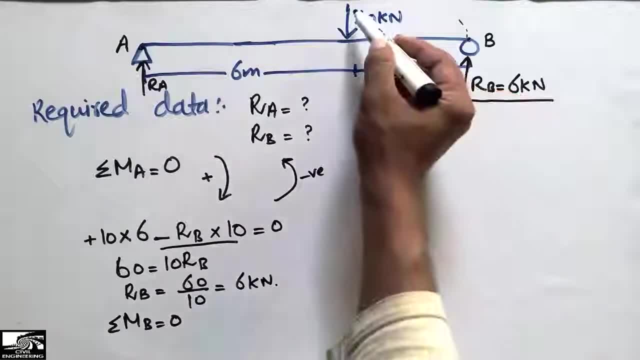 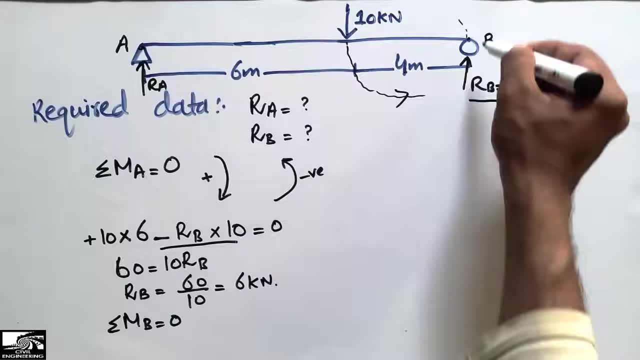 So the first one is the 10 kN for 16.. But now, in this case, you can see here it is acting anticlockwise direction in this direction. So it is the anticlockwise direction around the B point. 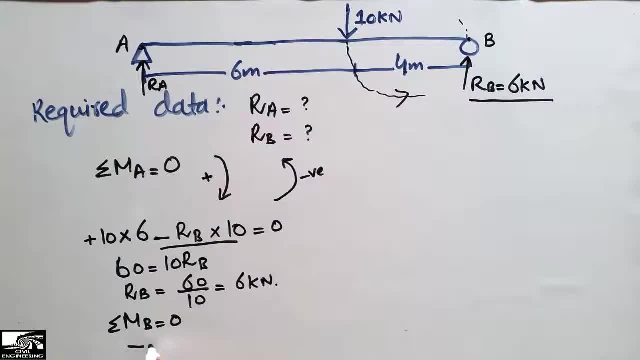 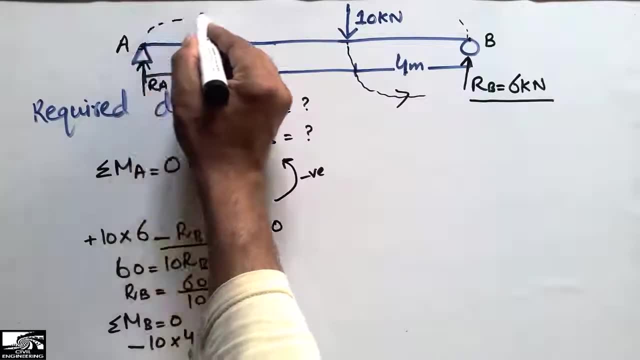 So in case of the anticlockwise direction, we can write it here with the negative sign Minus 10.. Into 4 m here, Then Ra, Ra. here is the clockwise direction. You can see here it is acting upward. 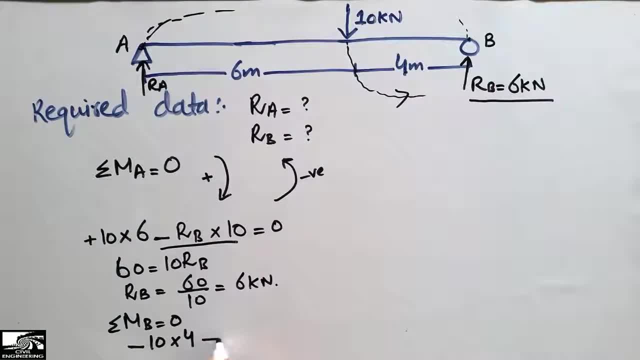 It is acting clockwise around the B point, So plus sign with Ra into the moment arm is 6 into 4.. 10 m is equal to 0.. Summation of moment is equal to 0.. Now we can write it here that 10 into 4 is 40. 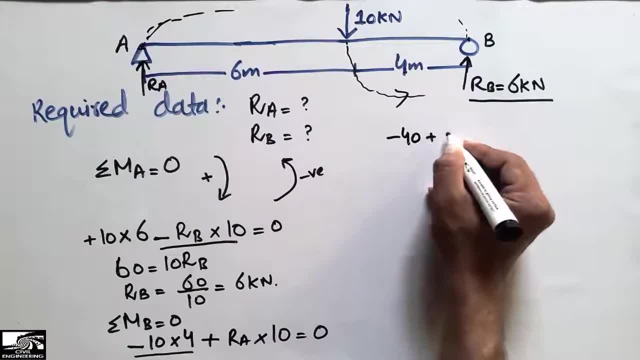 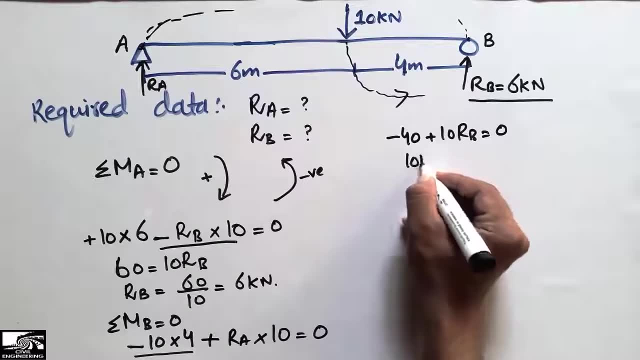 So negative 40. And plus 10. Rb is equal to 0.. So now we can transfer this into the right-hand side. So 10 Rb will be equal to 40. Or we can say: Rb is equal to 40 divided by 10.. 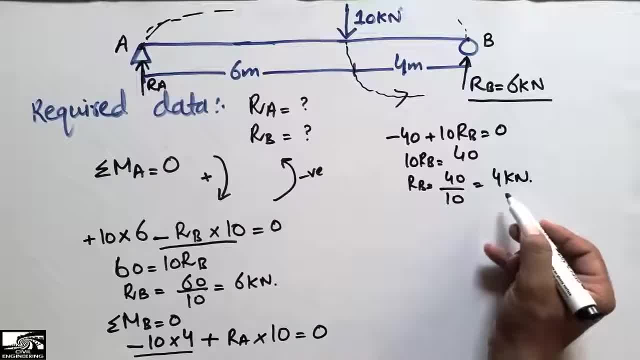 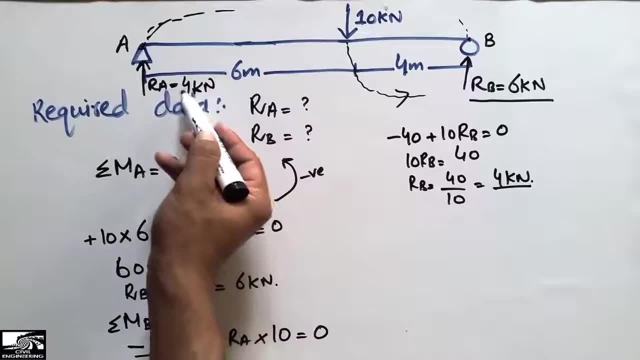 It comes out to be 4 kN, So it means that the Ra provides the 4 kN resistance to this concentrated load of 10 kN. The Ra provides less resistance- 10 to 4 kN- While Rb provides more resistance to the 10 kN load. 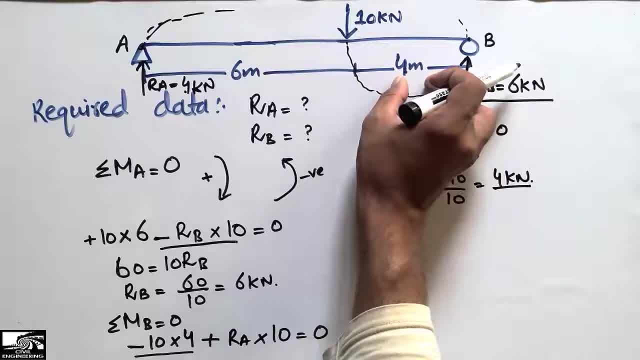 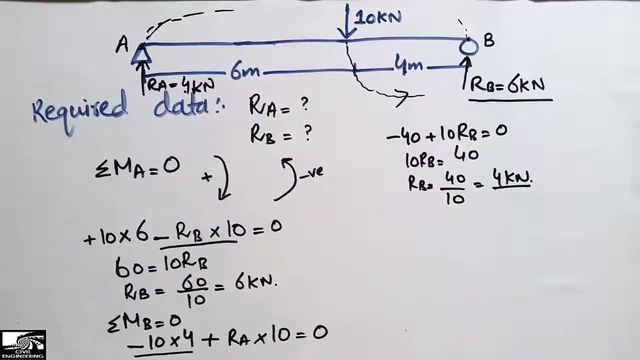 Because Rb is negative, So it is near to the load. It is 4 m distance from this load, While it is 6 m. So the more near the load is, the more resistance will be provided by the support.